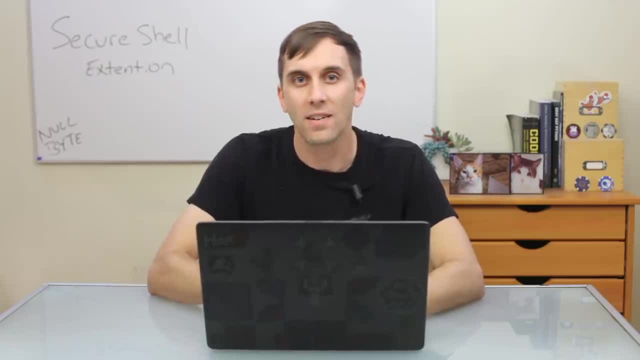 get into a terminal window in order to use it. In fact, some computers like Windows might not be able to do SSH from the terminal at all, and instead would need to download a third-party tool like PuTTY. Now, today, we'll show you how you. 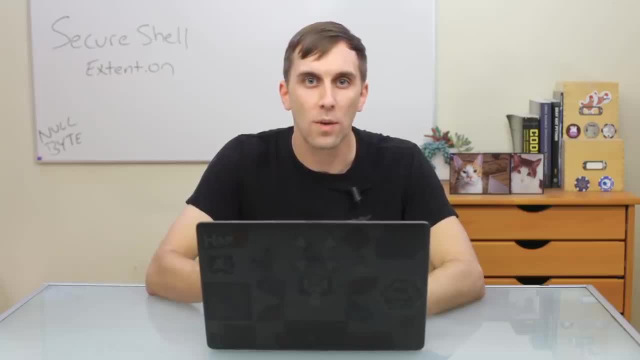 can avoid all this on any computer that has access to a browser window by using Chrome to download the Secure Shell extension. Now, what this does is implements a secure shell protocol within the browser, allowing you to connect to any device, either on a local network or on a far-flung network in. 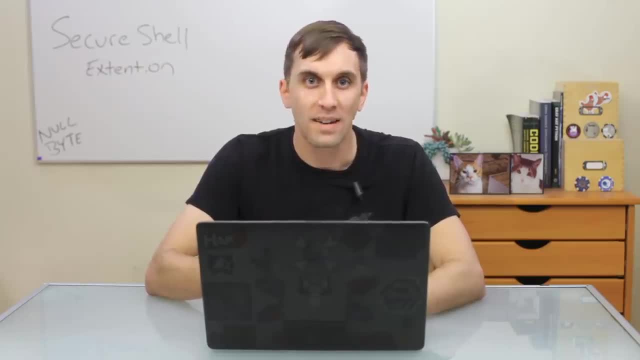 order to control it remotely via your browser window. Now, in order to do this, you'll only need to have Chrome installed, so this is a pretty easy one that everyone can participate in. Once you have Google Chrome, then we can begin. Now, before we get started attempting to connect to something with SSH, we'll need 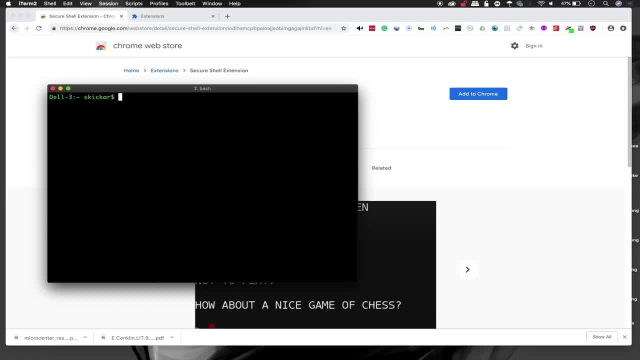 to actually find it on the network. Now, the two components of an SSH command are going to be the account we want to log into on the network, aka the administrator account or root or something like that, and then the IP address that the device we're looking to log into resides on, on the network or remotely. Now to find a 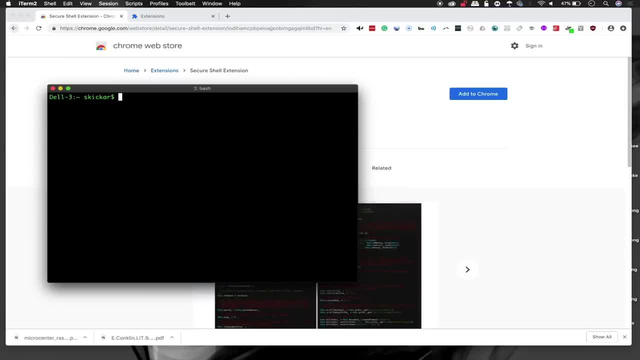 device on the network that has SSH. we can run a simple nmap scan, and I'll show you what we can do in order to locate any devices using port 22 as the default SSH port. Now, first we'll type sudo nmap and then tack p, and 22 is going to be the default. 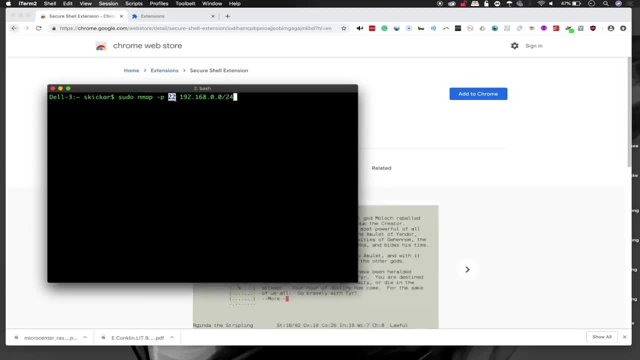 port that SSH runs on, unless you select a different one. Now, here we're going to assume that everything is running on port 22, and then we'll use the network range for this network, which in this case is 192.168.0.24.. If you want to find, 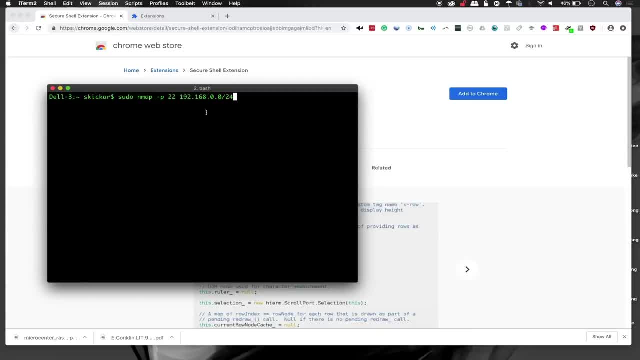 the network range on your network. you can take the IP address and just run it in IP calc, which will calculate the subnet for you, including calculating this nice little range here. So as soon as I run this then I should be able to see if there's any devices on. 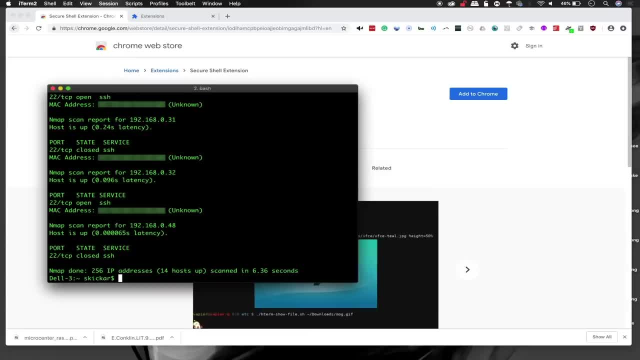 the network which say they have a port 22 open, telling us that that's one that we might be able to log into with SSH. Now here we are. we can see there is a actual port 22 open on 192.168.0.32. so this is what we'll be using today as our 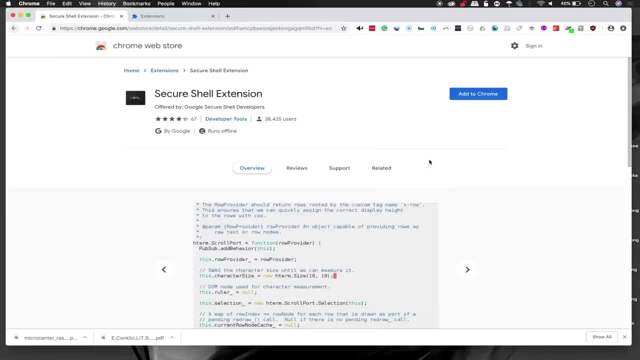 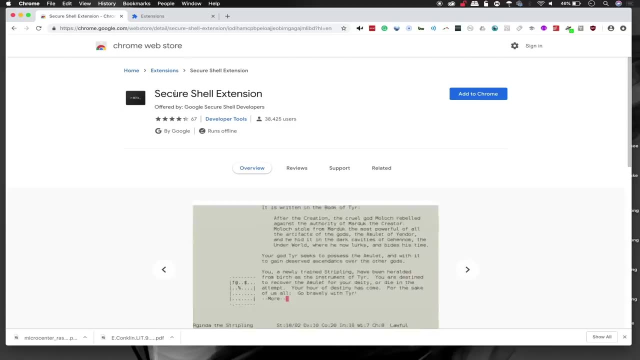 demonstration device to log into. Now, initially there's not much I can really do on just a Google Chrome window, but what we can start with is a little bit of a quick demo of what SSH is. So what we can start with is the secure shell. 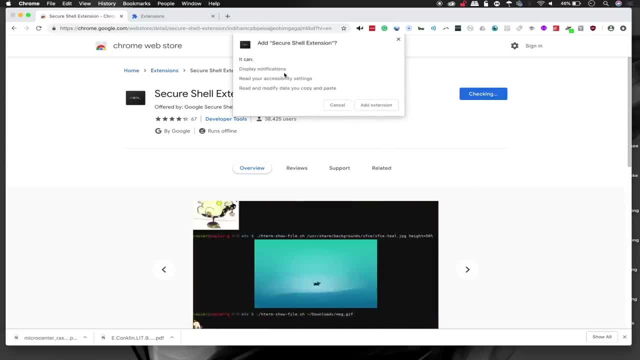 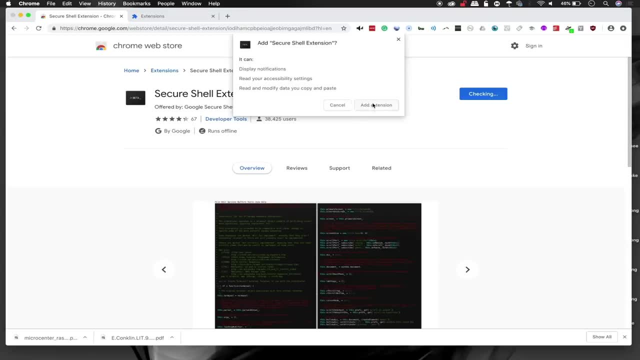 extension which is available in the Google Web Store. Now, when we add this to Chrome, it'll go ahead and ask us if we want to add the extension and we can see it can display notifications, read your accessibility settings and read and modify data you copy and paste. So we'll go ahead and add the extension and then. 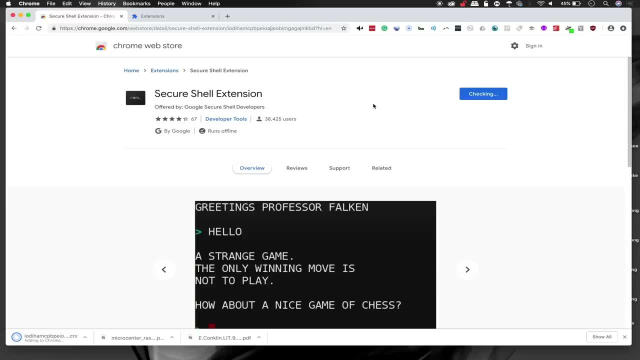 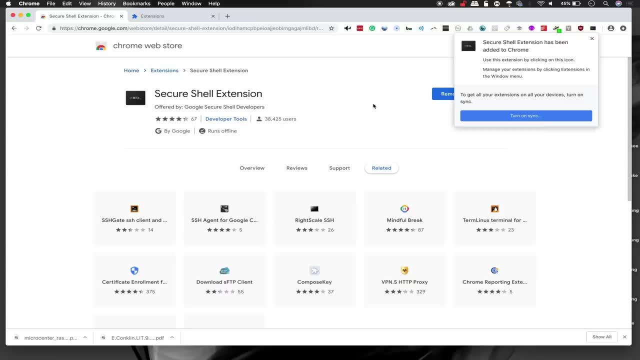 once we add that it should be relatively simple to log into devices on the network. Now we can go ahead and be more specific with this, and we can even go ahead and make it so we can even maybe remotely revoke that key in the event we want to disable somebody from breaking into our connection. Now I'm going to go. 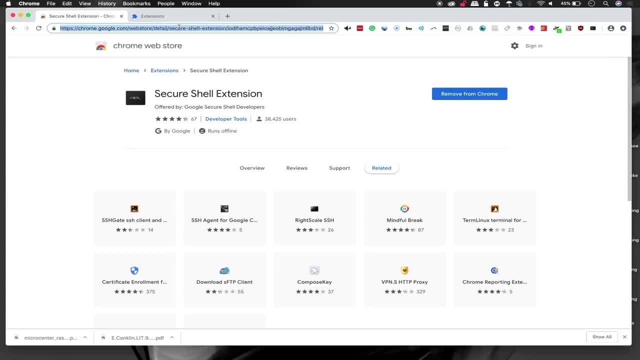 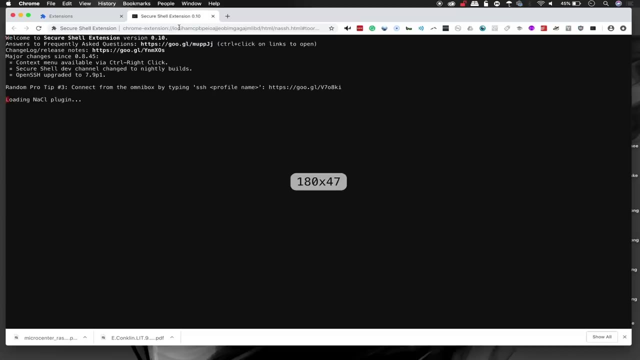 ahead and close out here and we see it's been loaded, so let's test it out and type SSH and then tour at 192.168.0.32.. So we're typing this in like it's a website. let's see what happens when we run it. Here we go, so we seem to get. 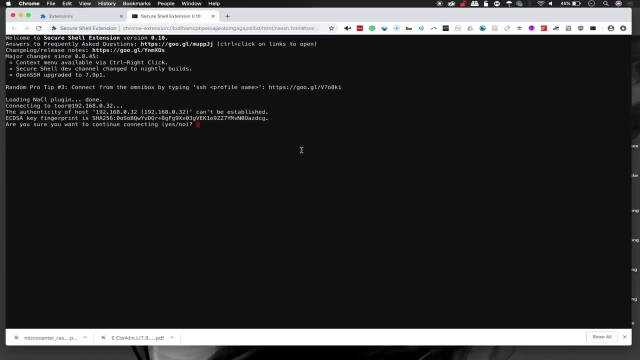 a shell, which is pretty cool to have available in the browser, and it's going to ask us the question about the authenticity of the host, and we'll need to accept this key if we want to connect Now. if this changes later, then it won't allow us to actually interact with this, so make sure that this is actually the 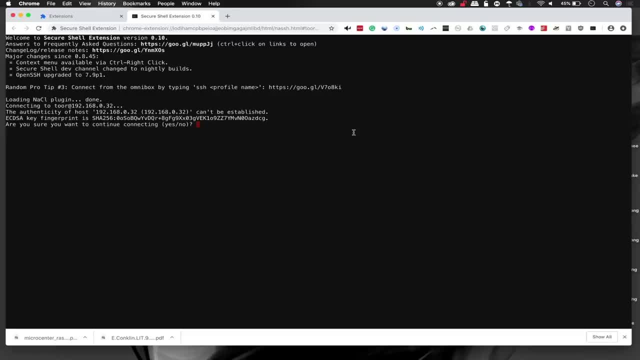 device that you want to connect to, before connecting to it and choosing to trust this key. In this case, I'll type yes, and now I'll get to the part where I need to supply the password and prove that I have permission to connect to this host. So I'll go ahead and click OK. 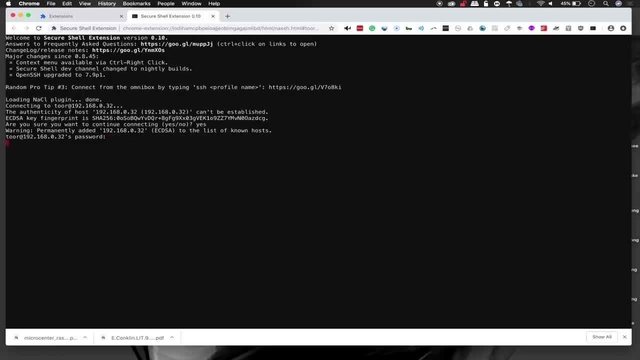 And here we go. we are actually logged into this Ubuntu device and now we can go ahead and do whatever we want. We can type ls, we can reboot it. all that is now available to us in this cool connection. So that's pretty interesting. but what? 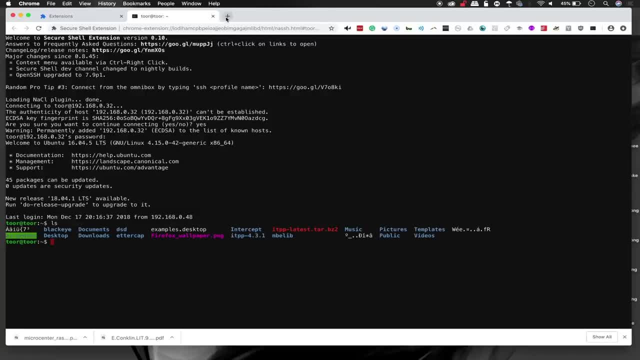 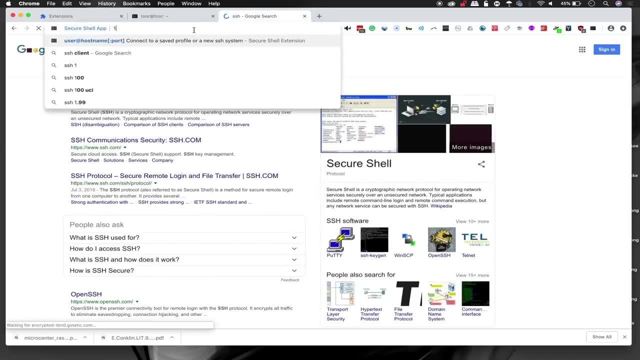 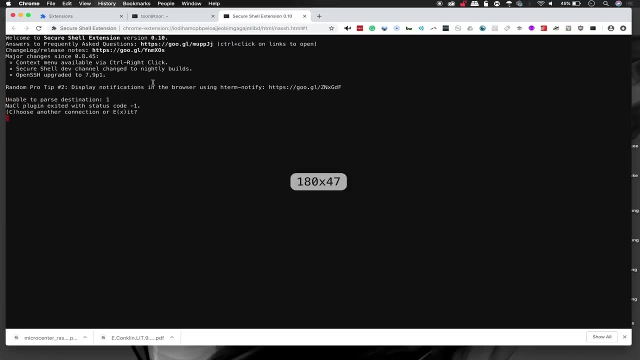 else can we do with SSH? So if I open a new window and then type SSH, I can go ahead and see I can hit the SecureShell app, and there's a couple different suggestions for how to do this. Now, if I want to type C for choose another connection, I 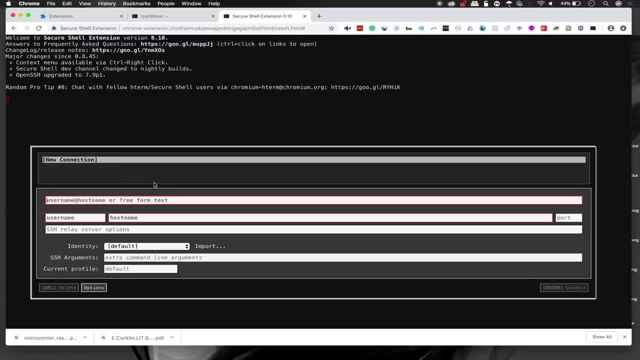 get this new connection window and I'm able to enter in all the information bit by bit and kind of be more specific about it if something's changed Now. an example of this might be if we're using a port other than 22 in order to avoid. 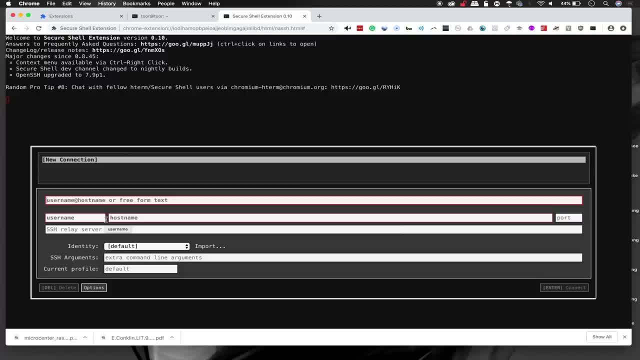 you know, scans like the one I just did. basically Somebody who wants to hide their connection might move it over to a random other port, maybe port 81 or port 222. really, whatever they want to do, they can move it to a different port and it would be a little bit harder to find on. 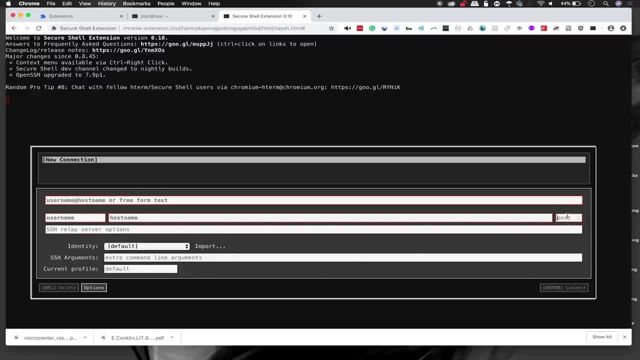 a typical scan, But here we can select a different port and type in, let's say, 222, and we can even go through and save different identities or add arguments to the SSH command in order to do other things other than just simply creating a direct connection. 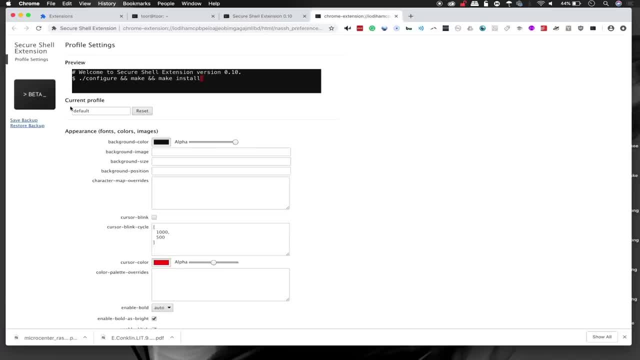 Now I can also use the SSH command in order to do other things other than just simply creating a direct connection. Now I can also click on the options and we do other things, like set up a profile, change our appearance and manage the app a little bit more thoroughly. but in general, this 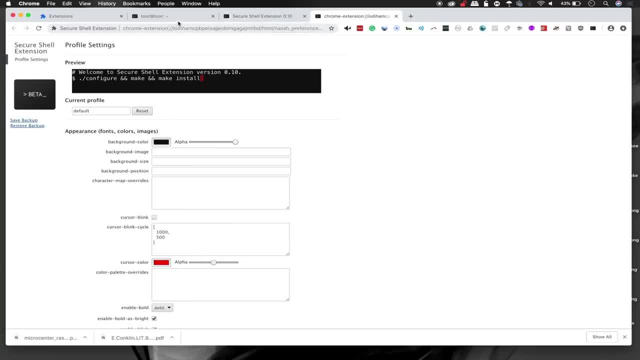 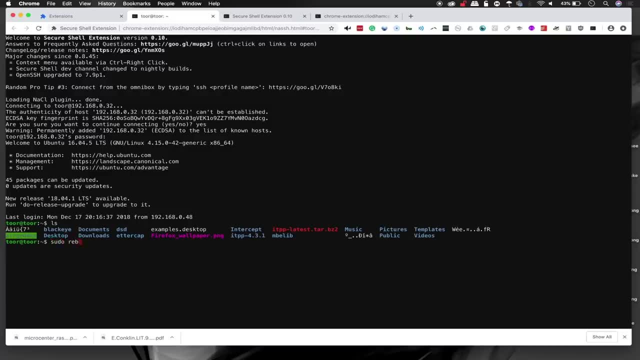 should be enough to execute whatever command we want on our system. Now just an example. I'm gonna run a quick command here and show what happens if we do a sudo reboot. We should be able to reboot the system remotely. and there we go: we get kicked out because we have executed command on a remote device from a. 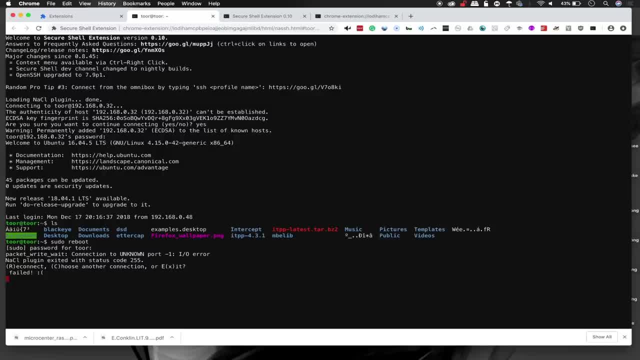 simple Chrome browser. Now, this extension is really useful and, of course, like I said, it can also be used for any devices, let's say, you discover on Shodan. but it's important to note that, while it is a secure shell, that doesn't mean that 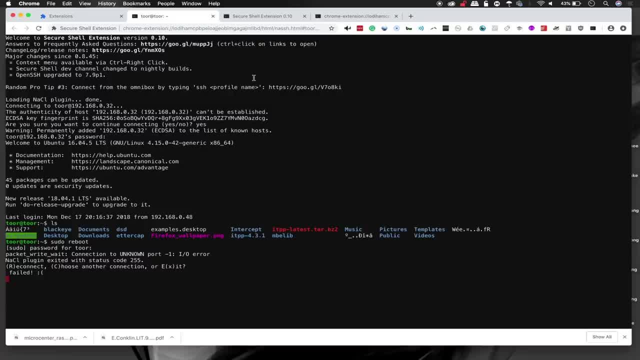 people can't see what you're doing, especially if you're attempting to connect from your IP address to their box remotely. Before you go about connecting to something that you don't know what it is, consider very carefully that SSH honeypots are extremely popular, so don't let that be a way to link your